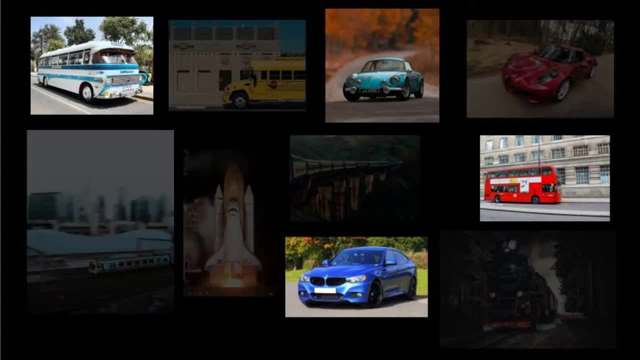 to point out which ones picture the bus. We can do this for a bunch of times and hopefully a ratio of correct and incorrect answers will favour the former. But if we just show it the same set of pictures of a bus and then some abruptly different systems, we can't get any answers correct. So 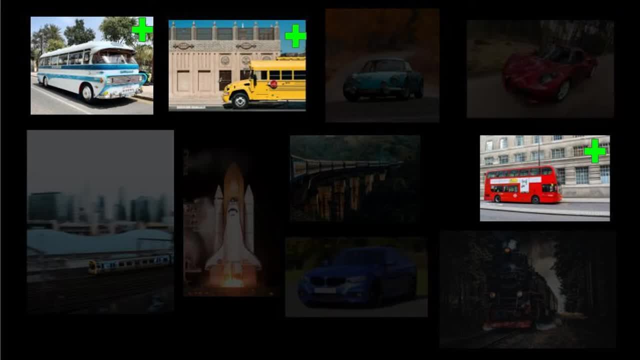 let's start with the first one, Because this is a very simple program. we need five pictures of a bus over and over again, then in the end it will simply remember the correct answers. In this case, we witness something that is called overfitting. It leads to a hundred percent. 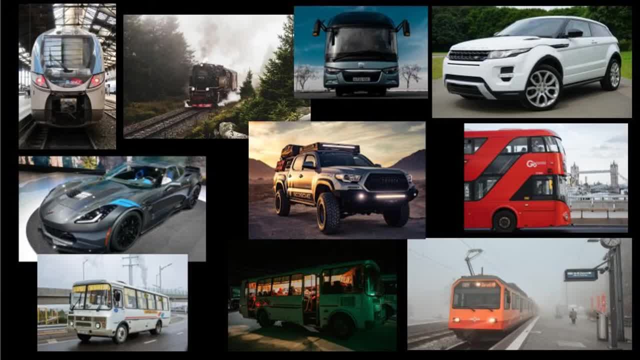 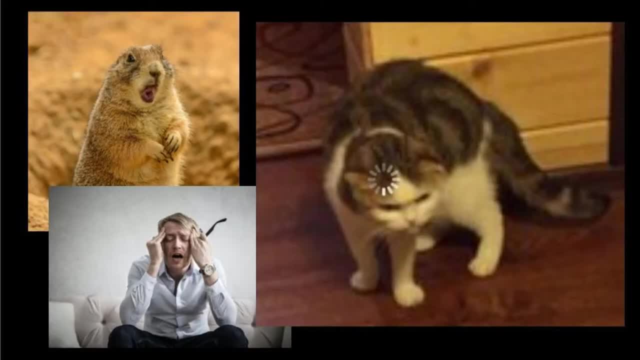 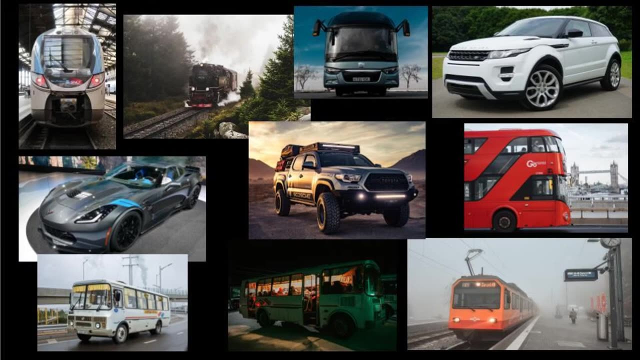 guess in accuracy for the data it was trained on. but when the model meets previously unseen data, it fails to generalize its knowledge onto new examples and therefore it fails altogether. Therefore it makes sense not to train our model on the entire data set at once, but to keep some parts of this data. 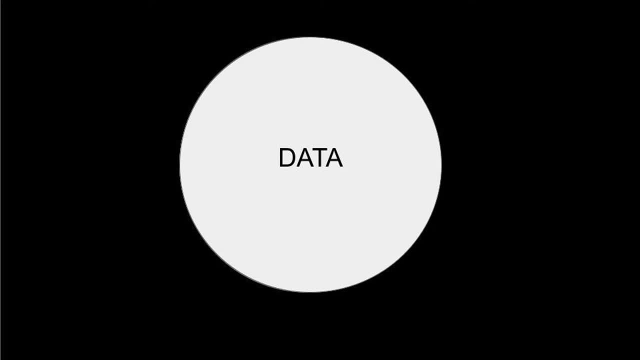 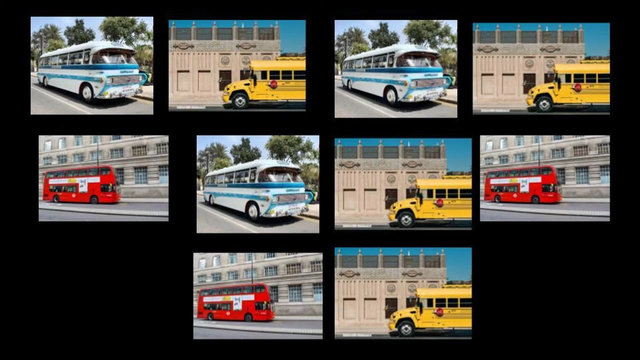 for later tests. In fact, we want to split our data set into three parts. The first one is called the training data set. This is the data on which we will train our model In the bus example. it can be a set of pictures that we show to our 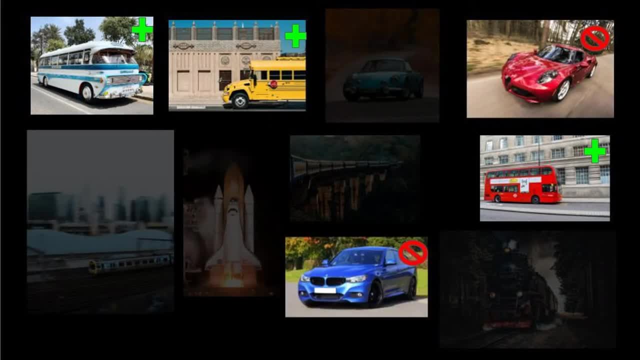 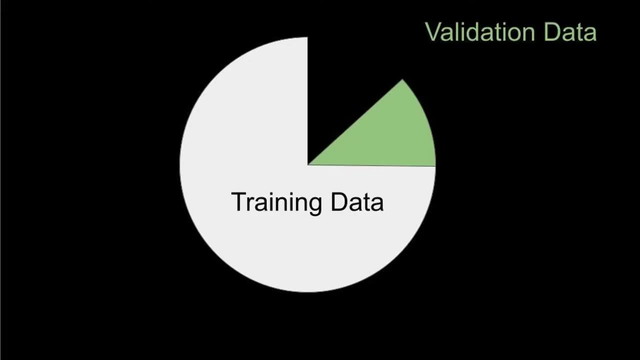 AI and we say something like: hey, this is a bus and this is not a bus, You understood? The second one is called the validation data set. This is a data set that our model did not see and therefore it cannot know in advance which 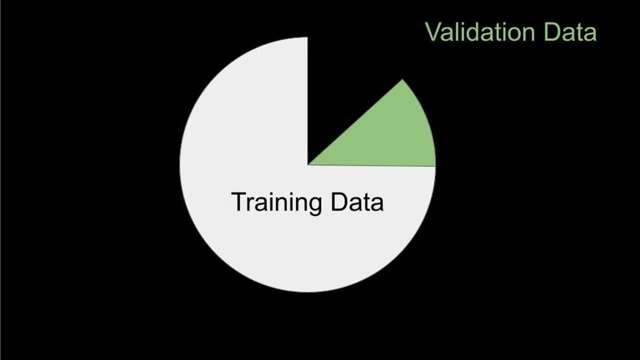 answers are correct and which are not. In fact, we'll try several different models or their hyperparameter values and, using such a validation set, we will determine which type of model or their hyperparameter values does the best job of identifying them. Finally, there is a test data set. This data set is necessary for an 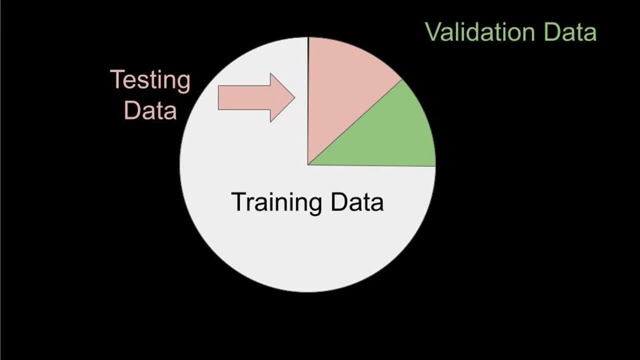 unbiased assessment of how the model will behave in a sort of real environment. In fact, this set is similar to the validation set. The model is also not familiar with the data in the test set and the only difference between them is that we'll use the validation set to find. 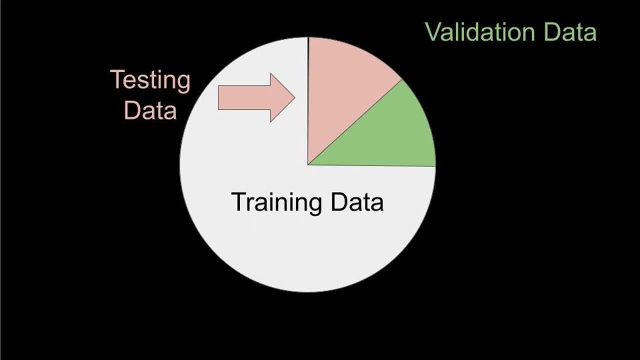 the most efficient model and a set of its hyperparameters, And then check on a test data set to make sure our chosen model still performs well. So the question is: how do you divide the data set? What are the proportions for training, validation and test sets? And the answer is: 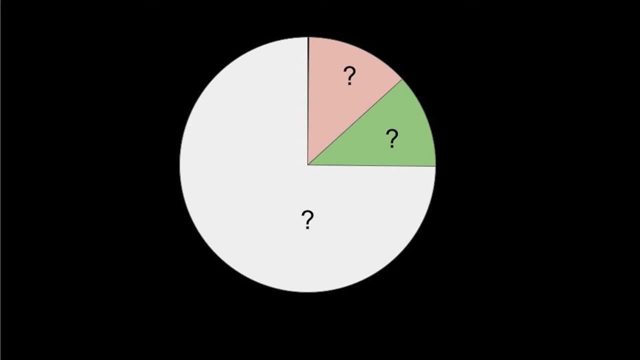 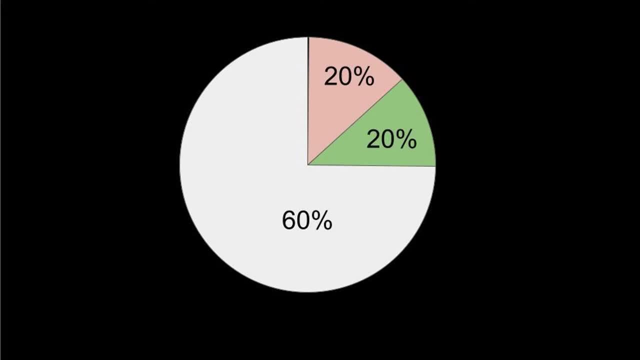 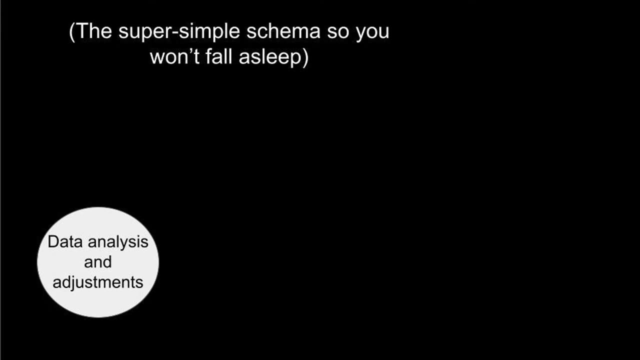 So let's start with the training set and 20% for the validation set. So let's start with the training set and 20% for the validation set. The whole process may look something like this: First we analyze our features, process, clean and optimize our data set. 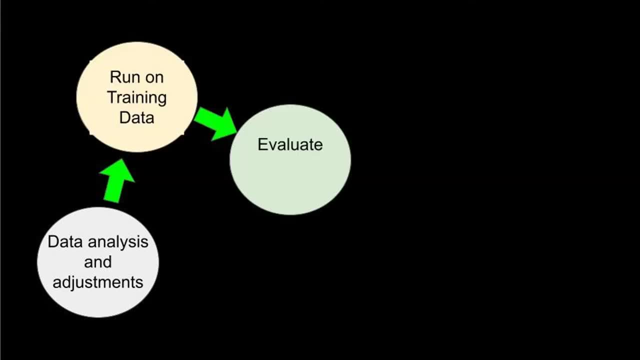 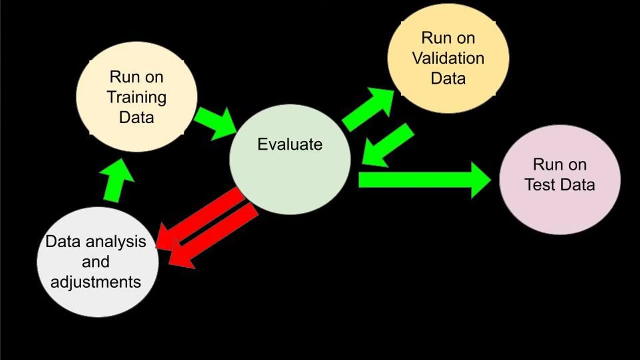 Next, we train the model on the training data, evaluate the result and, depending on the evaluation, decide whether we should do some more data preparations and training or move to the validation stage. After that, we should also need to decide, based on the evaluation of the results, whether we 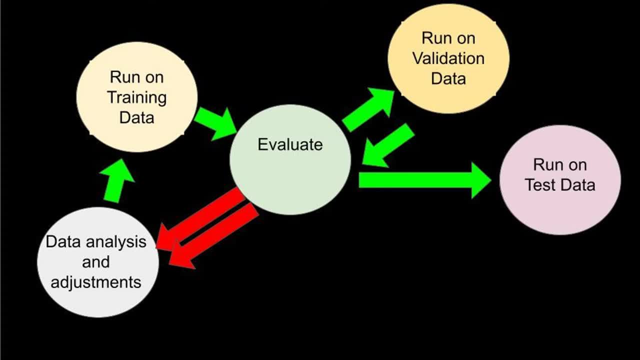 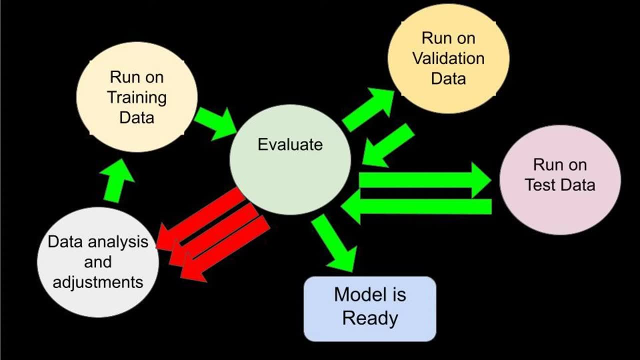 should take the best performing model and proceed to run it on the test set, or should we return to the training stage? And if the model performs well on the training set, then the model is pretty much ready. Otherwise, if the results on the test set are strikingly different from the results, 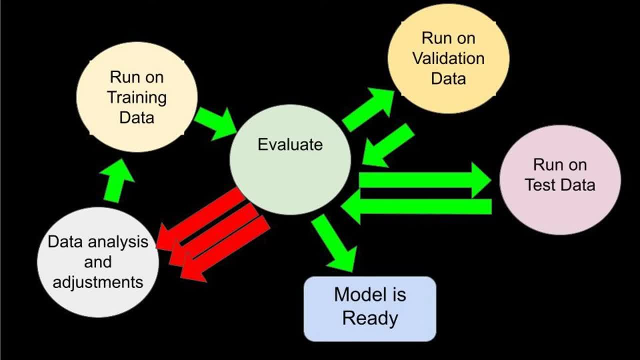 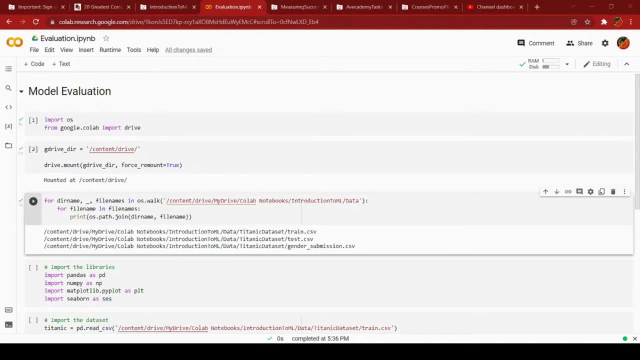 on the validation set, then we should roll back and investigate. All right, so now let's perform the split into training, test and validation sets. in practice. The only thing is, the Titanic, which we downloaded from Kaggle, is already split into training and test sets. But for the educational purposes we'll pretend. 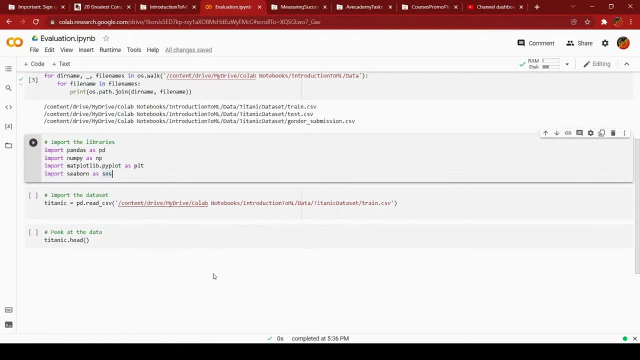 that traincsv is the only data set we've got and we'll perform our split on this data set. We are already familiar with this code from the previous lessons, so in that cell where we import the required libraries, we'll add another one called splitcsv. 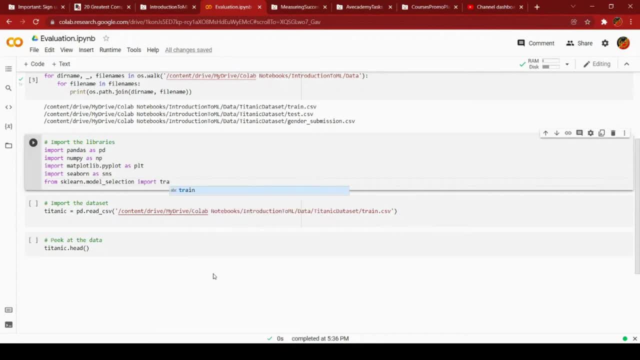 We'll call it scikit-learn or sklearn for short, And in particular we'll import the train to split from the model selection class And in the next cell we read the data set in csv format and we store it as a data frame in. 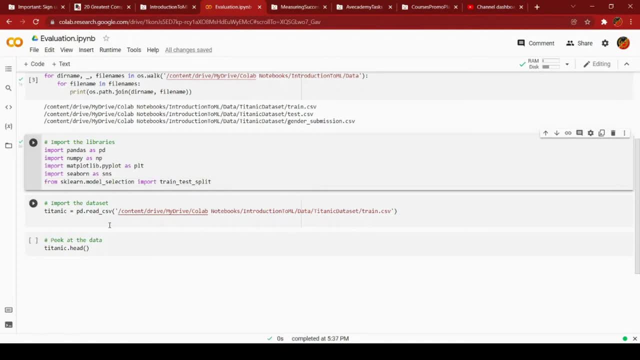 the Titanic Once again for this lesson. we are pretending that this is the only set of data we have And the last cell will just display the first five records. We're just going to have to figure out how to do that. So in the next lesson we're going to have to separate our data. 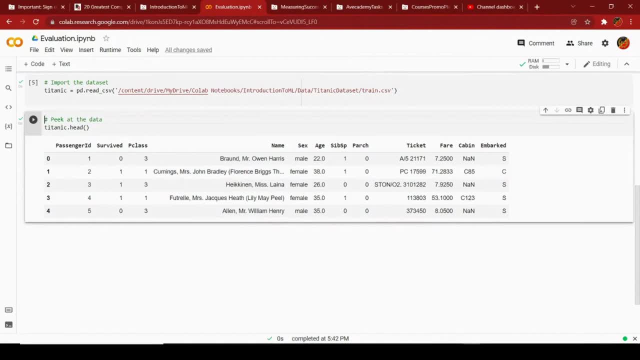 from the actual data set. So let's start by splitting the data into the table of the values of our data set. All right, And before we're going to split our data, we need to begin with splitting it into features and labels. 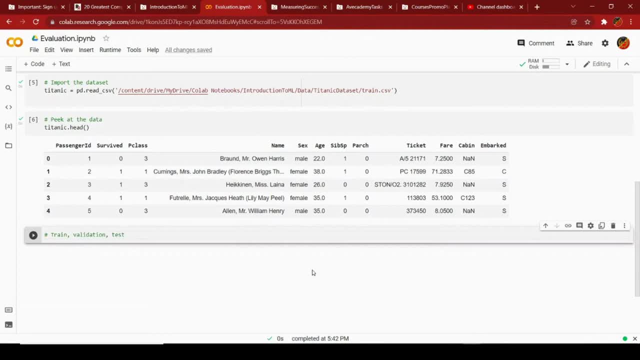 And it is pretty straightforward For features. what we need to do? we need to just drop the column survived, as this is our target variable, trying to predict whether a passenger survived or not. So we're going to declare two variables: features and labels. 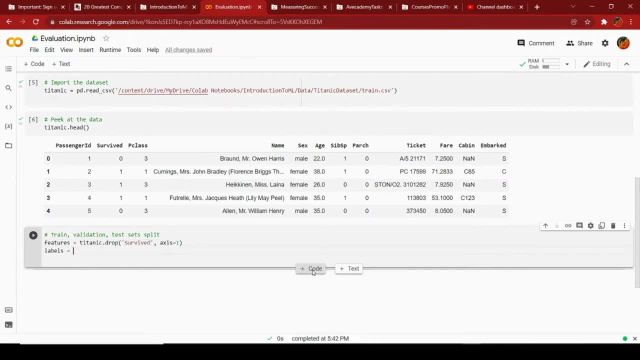 And for the features, we'll utilize the drop method on Titanic And we pass survived as an argument and axis equals 1 as a column. And then for labels, this is just the column survived And we'll need these features and labels as parameters. 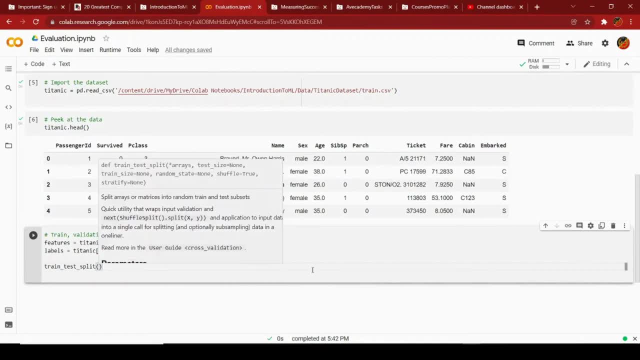 to our train test split method. So we need to pass features, then labels and then we need to specify the test size. Test size represents the proportion of the data set to be included in the test split, In other words, how much data we want. 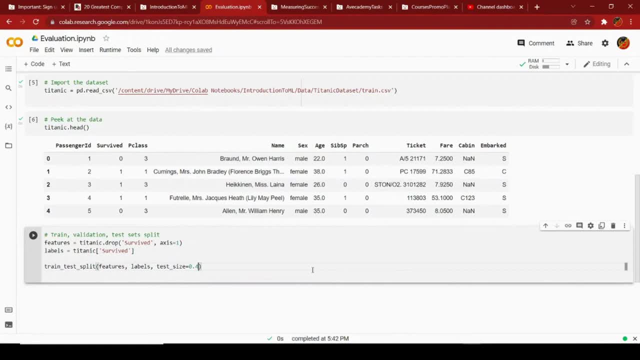 to reserve into the test and validation sets. But because train test split method can only split our data set into two, we'll have to perform it twice. Therefore, the first split will reserve 60% for training set and then 40% for training. 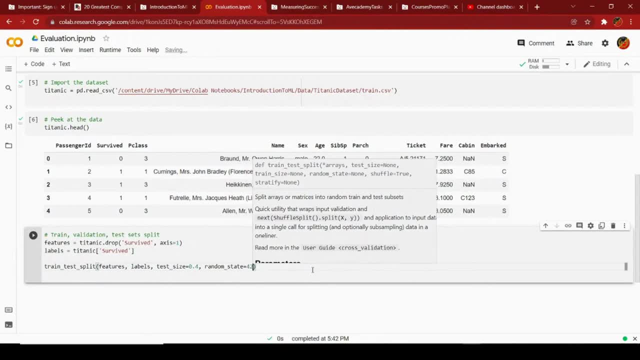 And then 40% for validation, plus the test set, And this random state parameter controls the shuffling applied to the data. You can read more on that in the official sklearn docs And of course we'll need to specify where we want to store the output. 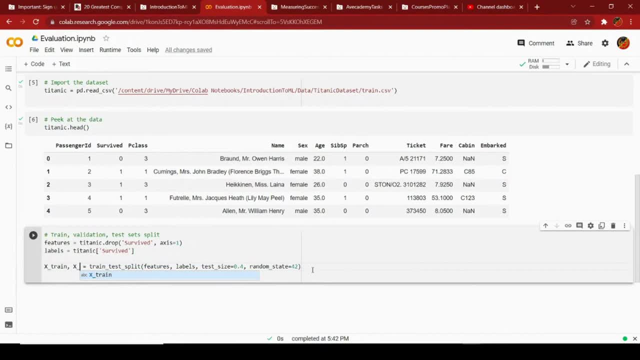 And this method has a predefined output order which we must follow. So, first of all, it takes our features and split them into train and test set, marked here with x. And then it does The same with labels, splits them into train and test set. 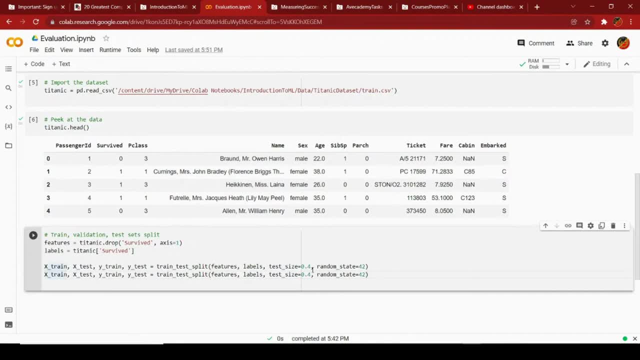 And this is the conventional representation of the outputs as it is specified in the official docs. And now, because of the train test split limitations I've mentioned earlier, we need to split our test set into the validation and the actual test set. So essentially I'm taking x test and y test outputs. 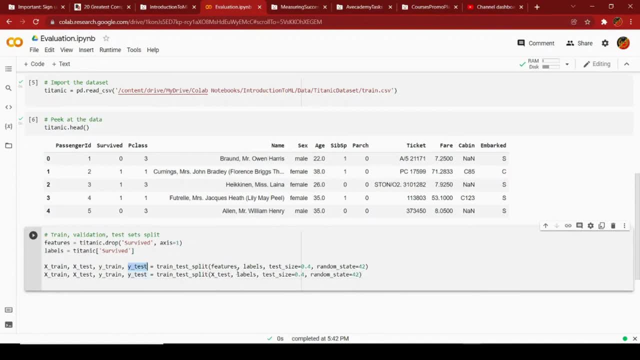 from the first call of this train And I'm going to call this train test split function, And these data sets will be passed as input arguments to this train test split function for the second call. That will split them half and half. Therefore, we'll need to change the value of the test size. 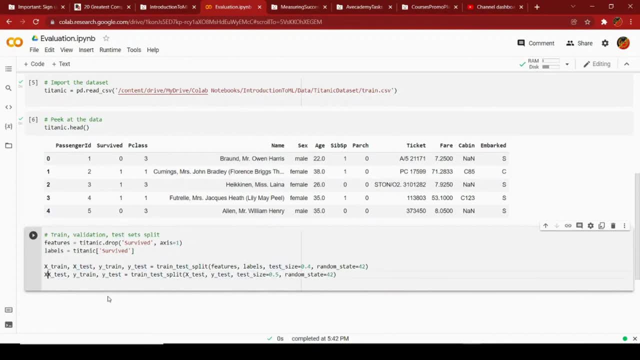 parameter to 0.5.. And we'll leave the random state as it is. So the only thing that is left to do is to change the names of the output data sets to xtest, xval, ytest and yval. 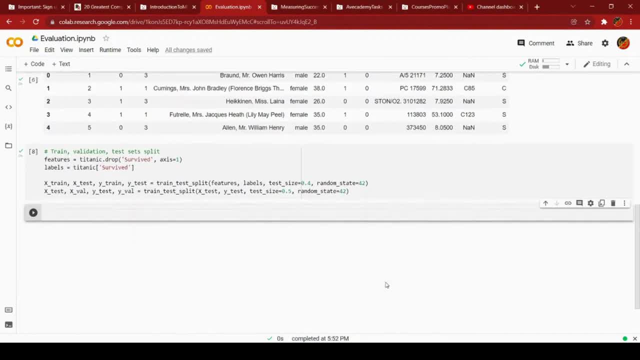 In other words, we use this train test split function twice to split our data into training test and validation sets, And after that we can check the data allocation by printing the length or length of these corresponding data sets. Labels will represent our full data set. 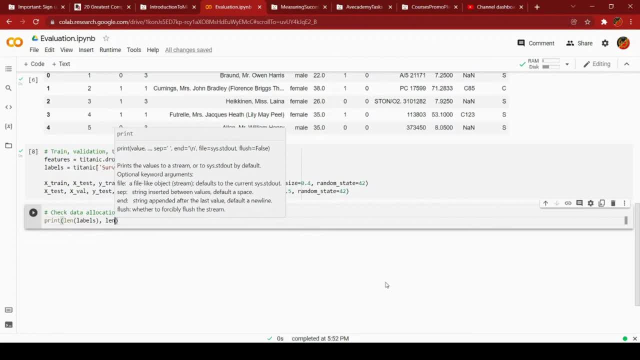 As you remember, the Titanic data set was already split into train and test sets And we were pretending that train data is the only data we have. so we're splitting the training data. labels represent the whole data set, this training data and then y train represents the training data set when we use the train test. 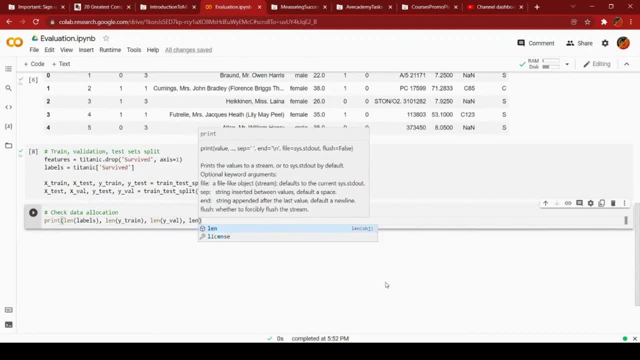 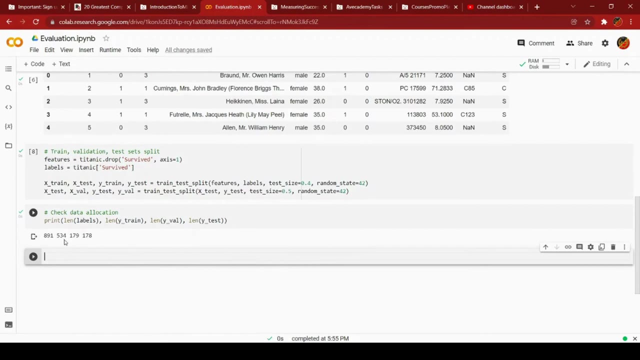 split for the first time. that should be 60 of our data, and y val and y test represent the second train test split 50: 50. they represent our validation and test sets and, as you can see, they had odd number of records in them. therefore they've been split that way. but other than that, 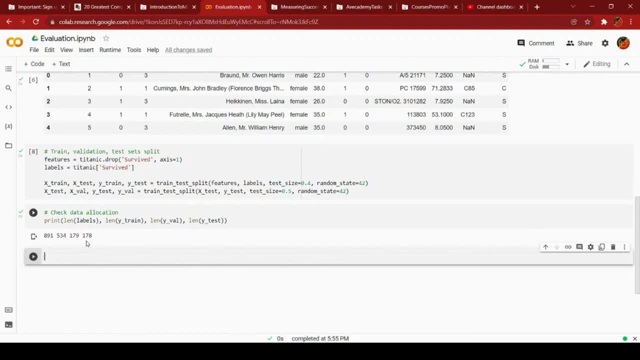 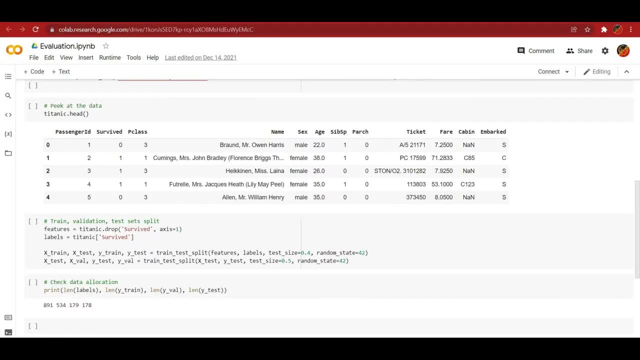 numbers do add up. if you have any questions, please leave them in the comment section or refer to the official documentation. let's continue with the concept of data holdout. so what we just did, we retained some of the data we're not going to use to train our model. 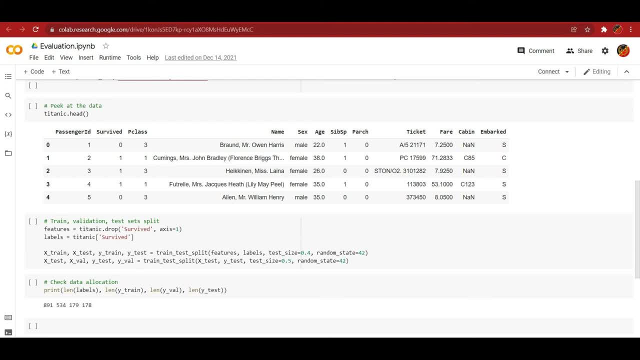 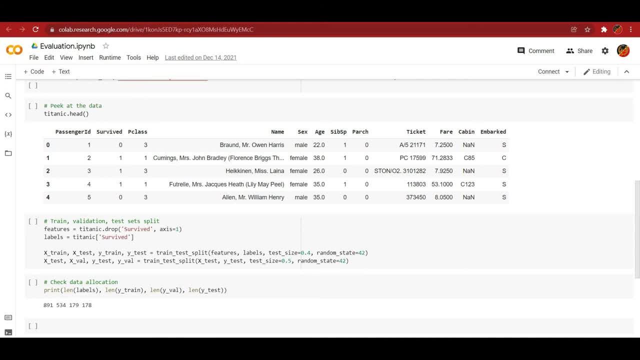 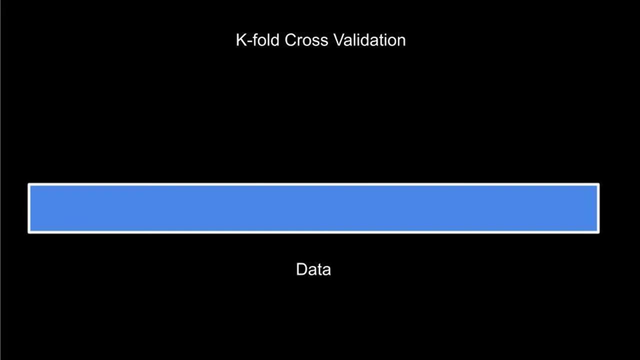 if we want to split this set again, we need to call the method again or wrap a cleverly written loop around it. however, there are many other methods for holding out the data, and one of them is called k-fault cross validation. it splits the data into k randomly selected subsets of 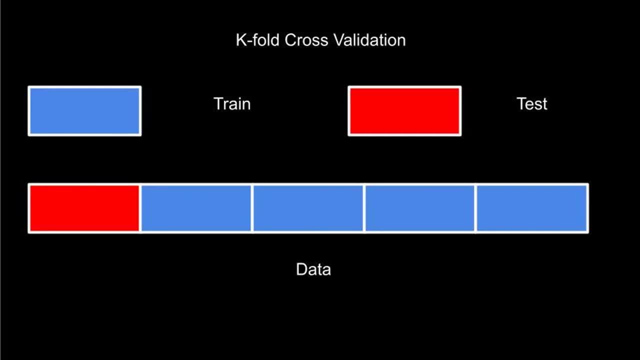 roughly the same size. one subset is called k-fault- cross validation- and it's called k-fault- is used to test the model and the rest are used to train it, and the trick is that if we divided our data into, say, five subsets, then training and verification will occur five times. after that we 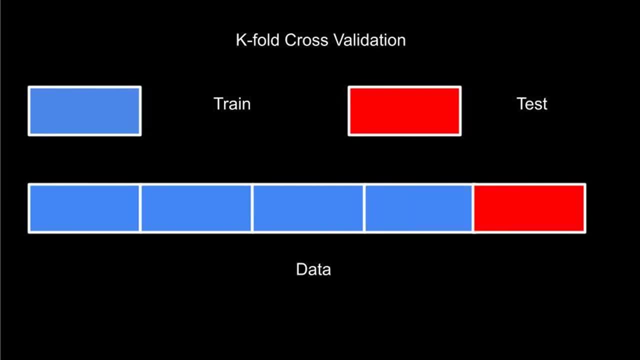 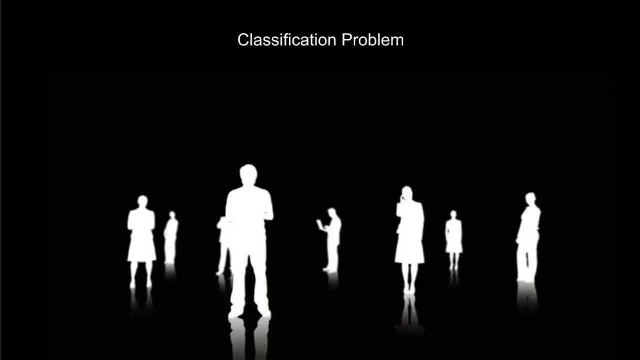 take the average of all five runs. and that brings us to another important topic: evaluation of the effectiveness of our model. we need a metric to understand how well our model performs, and here are some metrics at our disposal. in the case of the titanic, we are solving this so-called classification. 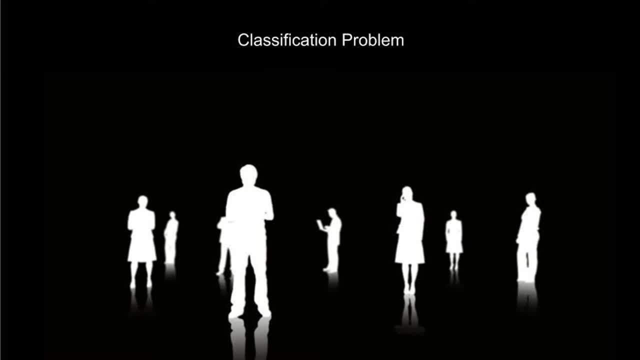 problem, that is, we need to determine whether the passenger will survive or not. zero, the passenger went under and one for a good swim with a happy ending. therefore, for the classification problem, we'll turn to classical metrics such as accuracy, precision and recall. accuracy is the number of 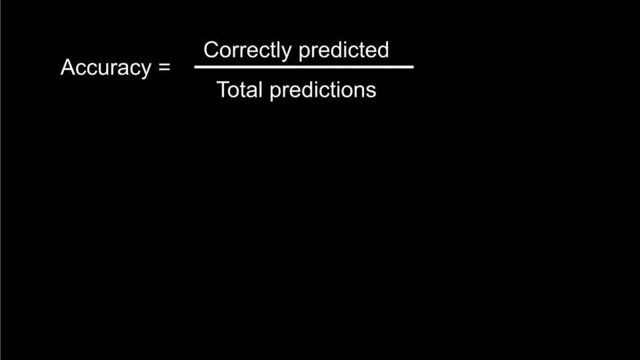 accuracy, precision and recall. accuracy is the number of correctly predicted outcomes for passengers on board over the total number of passengers on board. this metric has one interesting caveat: it assigns the same weight to all observations. this can have negative consequences if the distribution in the sample is biased towards a certain class, but don't worry. 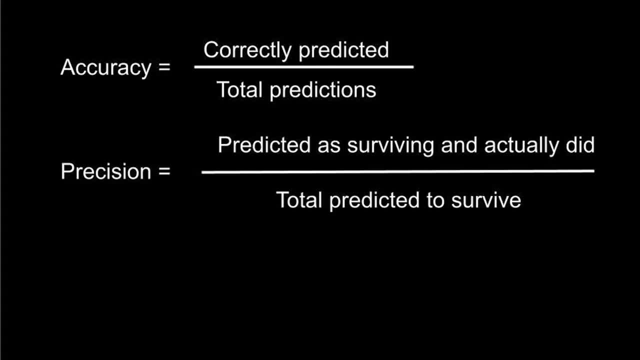 about it just yet. next one is precision. this is the ratio of true positives over the actual results or, in our case, the number of passengers who were predicted that they would survive the shipwreck and they actually did, over the total number of positive predictions. these include true and false.